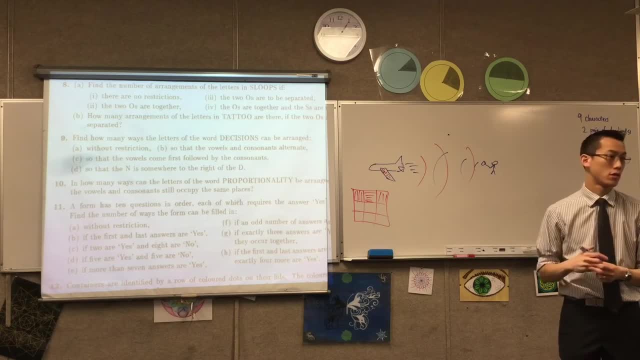 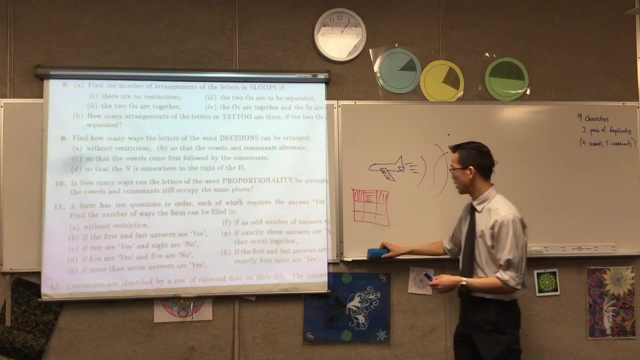 is that I believe there are four vowels and five consonants. OK, so let's just jot that down. That's not always important, but in this question it is, And thankfully no letter Y. OK, now let's just have a look at this really general question. 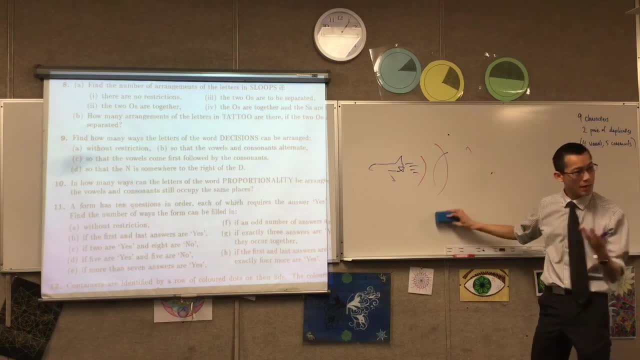 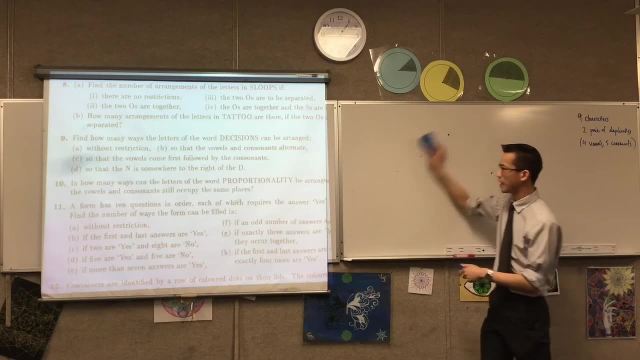 Secondly, at the beginning. firstly, how many ways can we arrange this word? and there are no conditions, no restrictions associated with it. So all of the information that we need is up here. It's only in the first two lines, in fact. 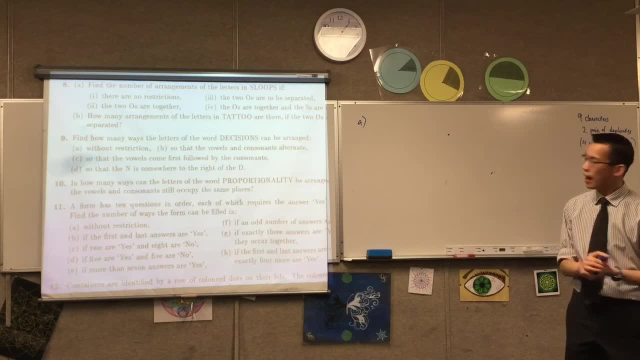 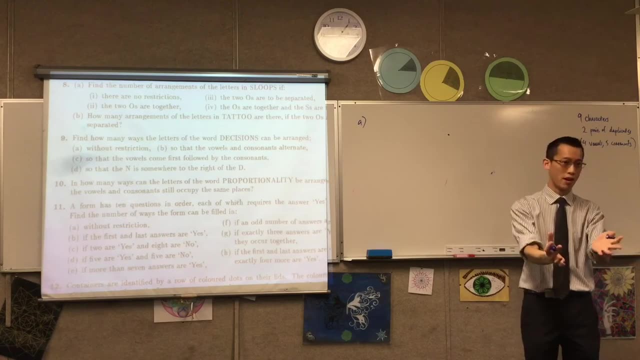 For part A and, by the way, as we break this down, I like to sometimes have a look at parts of the question: first, ways to do this, ways to do that, and then I summarise that by saying, OK, total ways. 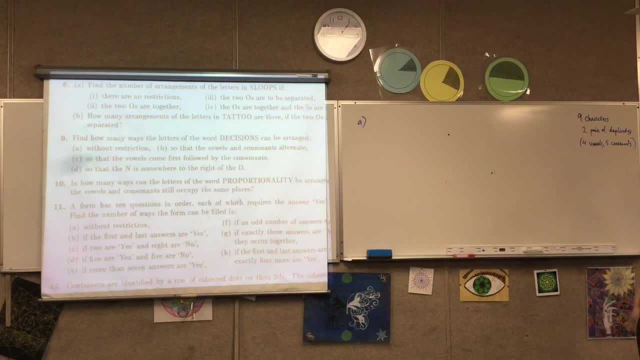 In this case. for this first one, you could go straight to the total ways, like there's not that much sort of extra subsidiary thinking required, So I'm going to write down total ways, No restriction. How am I going to do this? Can you talk me through what kind of numbers I'm going to need? 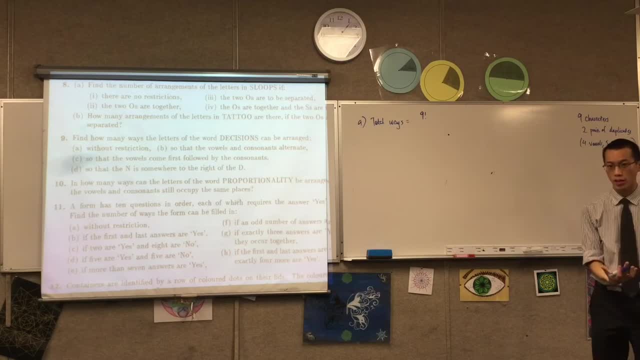 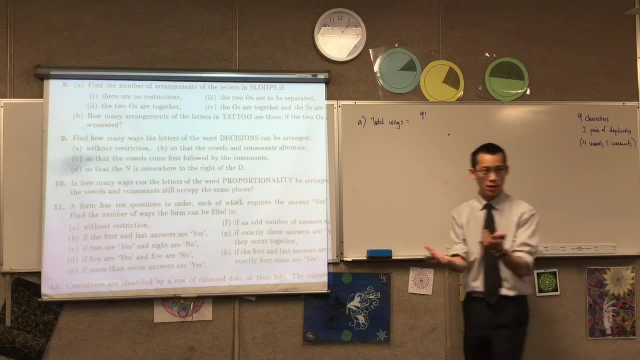 OK, so the start is 9- factorial. Now you could alternatively have said 9P9.. OK, I know I'm using P not C, because Because order matters, Because order matters. but how do I know that order mattered? Because it's a word. 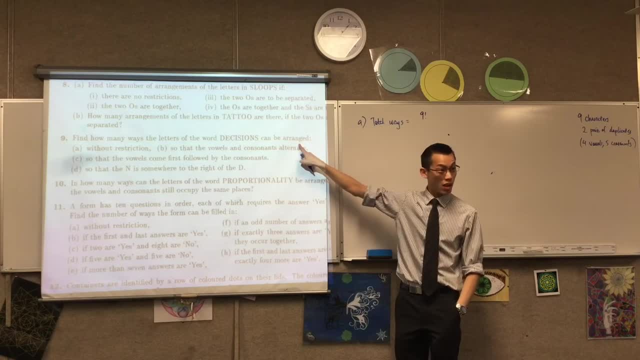 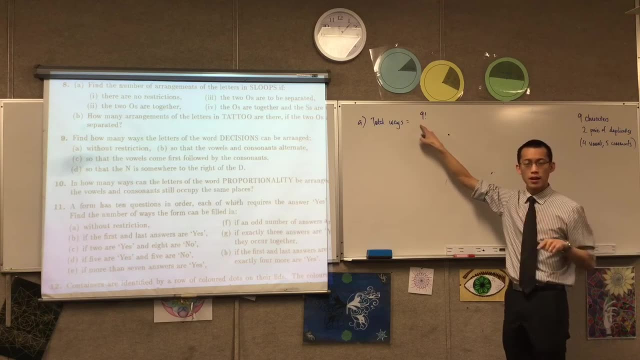 It can be arranged. Oh right, Look for that keyword. OK, So very good. So I could have used 9P9, but 9P9 is 9 factorial on 9. take away 9 factorial, That denominator becomes 1.. We saw that yesterday. 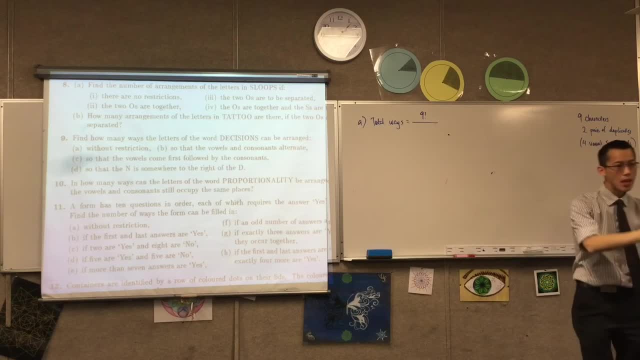 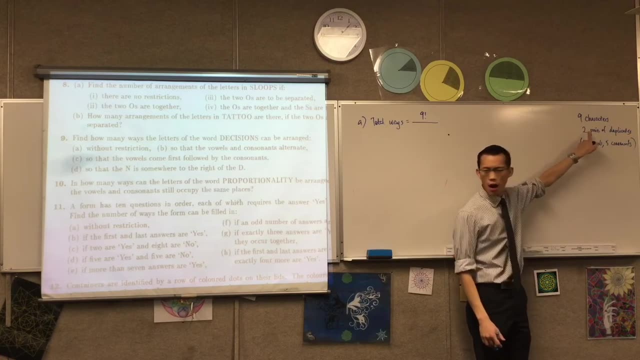 So I can just write it as 9: factorial. That's fine, But I've overcounted, haven't I? Because of the duplicate letters, right? So I've overcounted for the I's, Is it the I's? 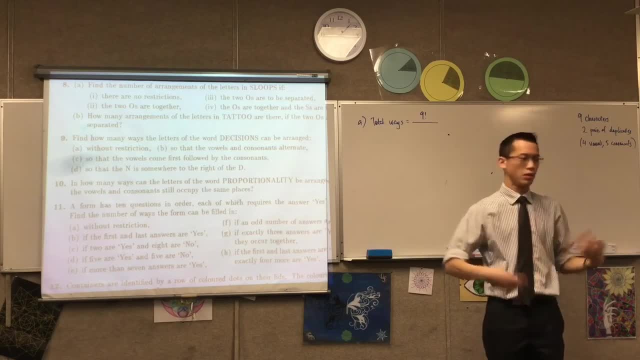 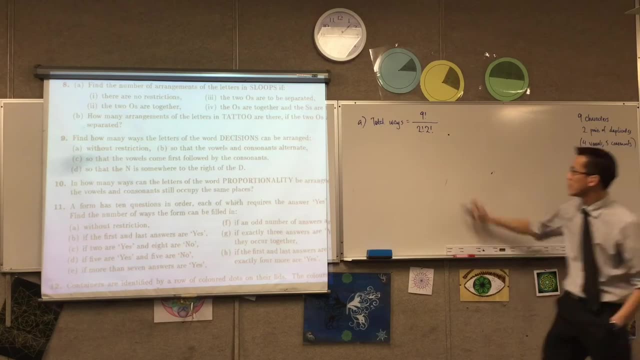 And I've overcounted for the S's because I can swap both of them and it looks exactly the same. So what am I going to have on my denominator here And I'm done? OK, Now I believe this number comes out to 90,720. 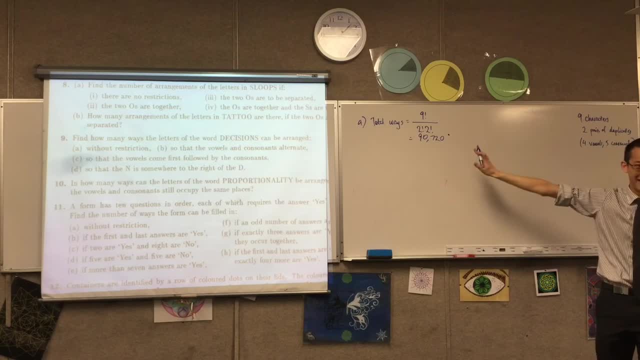 We'll point out that number doesn't really matter, It's this. This is what we look at. OK, So far, so good. Alright, now part B. It says: Find out how many ways The letters of the word decisions can be arranged so that the vowels and consonants alternate. 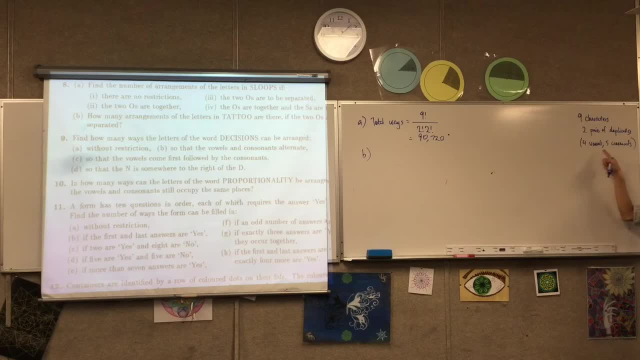 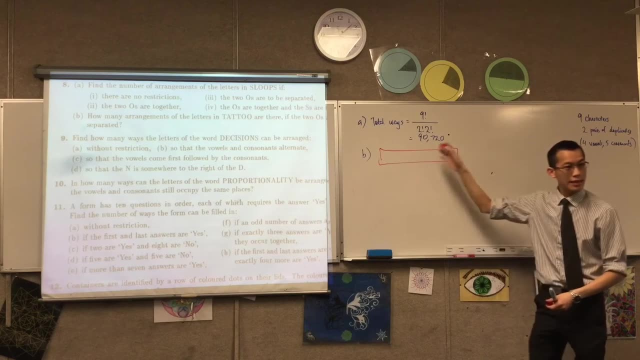 OK, Now have a look. You've got 4 vowels and 5 consonants, OK. So what this means- and maybe you want to draw this for yourself- is that, if you think about your 9 letters in sequence- right. 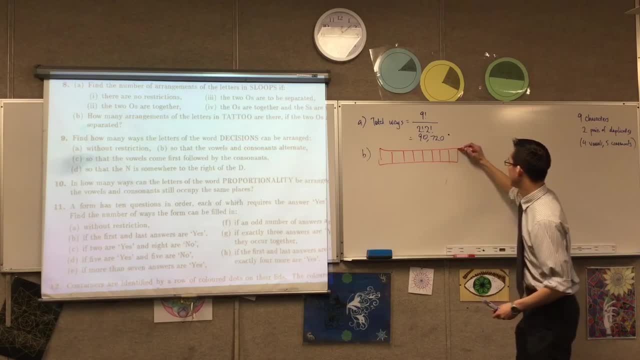 Oh, I've got enough. 2,, 4,, 6, yeah, last one. OK, if I want them to alternate, right? Do I get a choice as to whether I start with a vowel or a consonant? No, not. 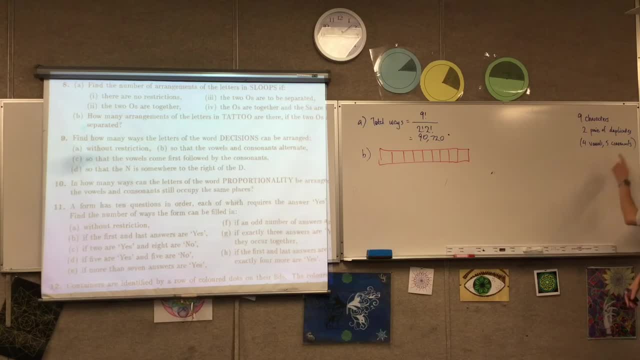 I don't really get to choose. I mean, I can choose which one, but I actually must start with a consonant because, of course, if I start with a vowel, I will run out of vowels and there will be 2 consonants stuck together at the end. 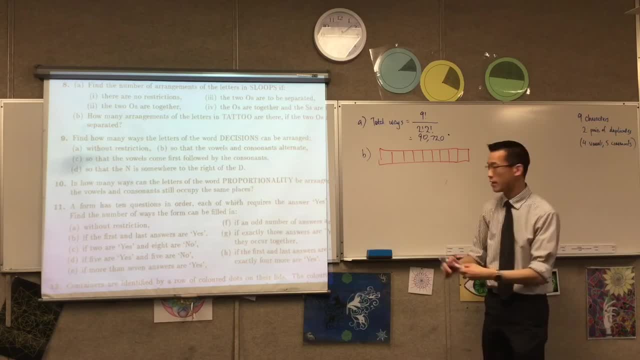 Does that make sense? So, therefore, when I look at this, the first thing I'm going to jot down is: this must start with a consonant, then a vowel, then a consonant, then a vowel, and so on. OK, 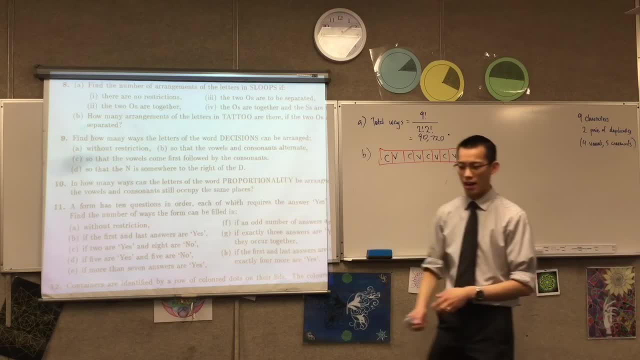 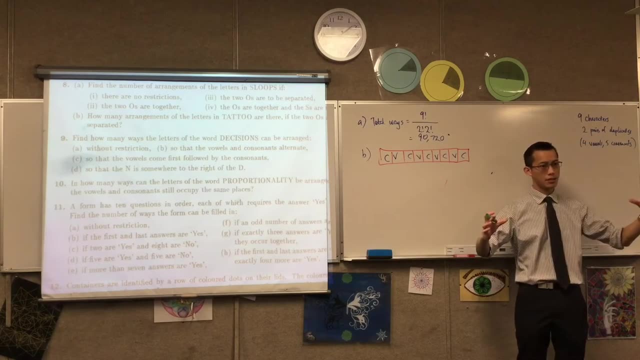 Does that make sense? Now? in a similar way to how I showed you with the blocks right, I'm now going to consider this as actually not one sequence of letters, but 2 sequences of letters that are kind of doing their own thing, right? 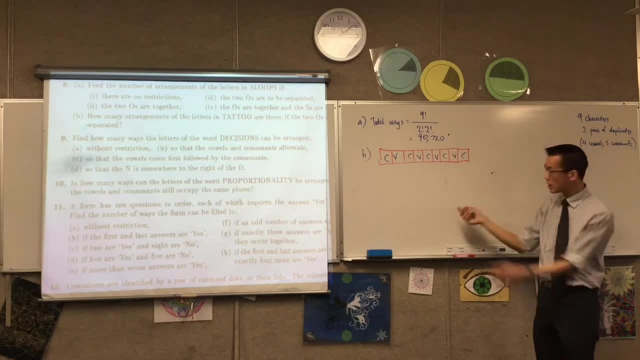 So what I'm going to do is I'm going to take out all of the consonants first. You see, they must occupy those spots. They have to be there. So I'm now going to say, Alright, poor guy, I'm going to pull them off to the side. 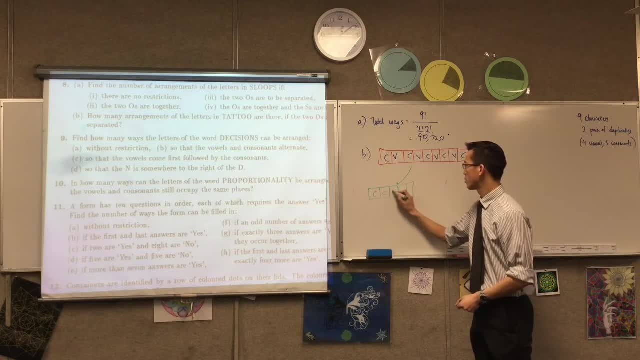 1,, 2,, 3, 4.. There are 1,, 2,, 3,, 4,, 5.. 5 consonants and they'll be in some order, right? How many ways are there to arrange these guys? 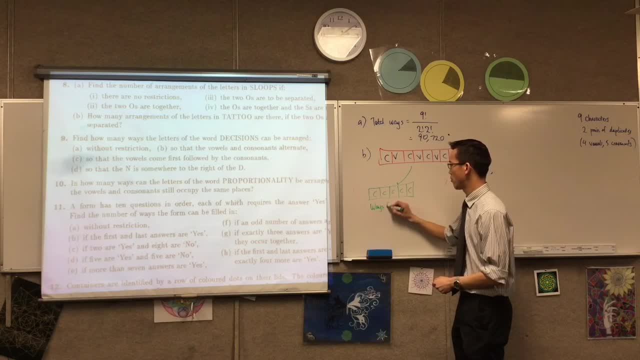 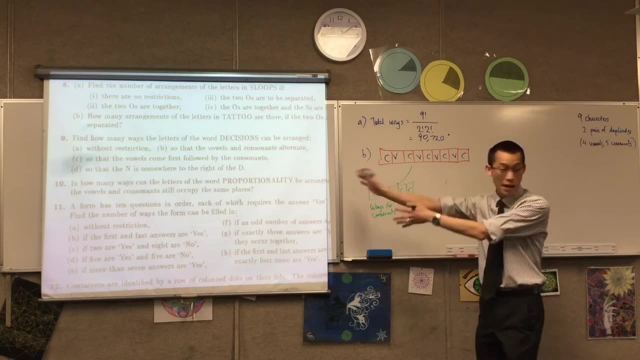 OK, good, So ways for So all of this stuff on your piece of paper. that'll all be about question D, OK, so we're just sort of setting up the beginning, right. So the ways for the consonants. here it's 5 things into 5 spots. 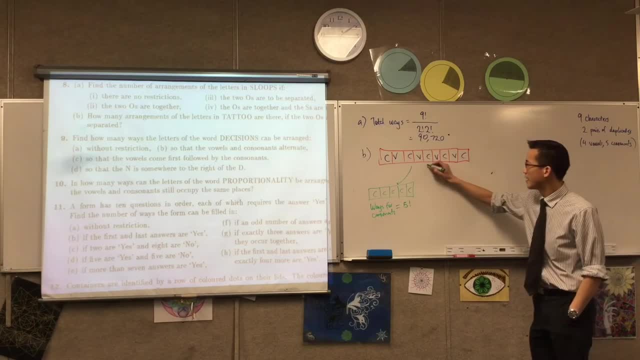 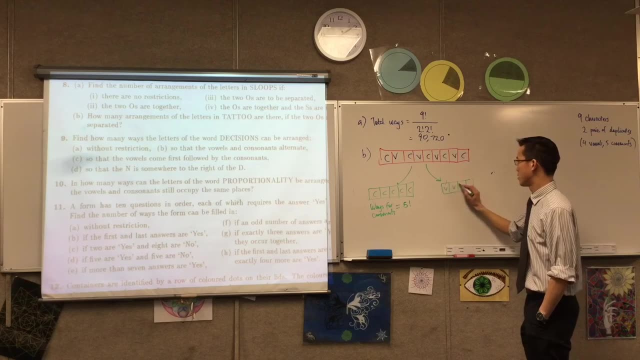 So it's 5 factorial, OK, And in the same way, I have to arrange the vowels right. There are 4 of them. Good morning, Grab a seat, take a piece of paper. So the ways for the vowels. 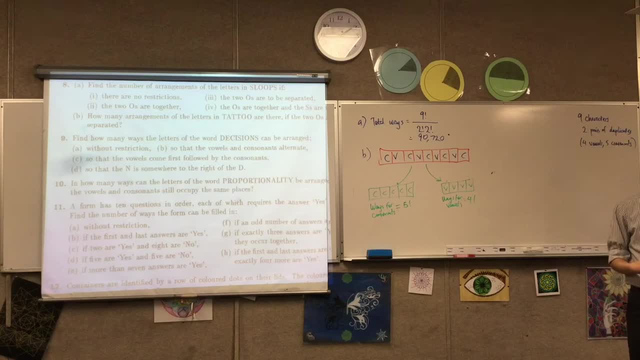 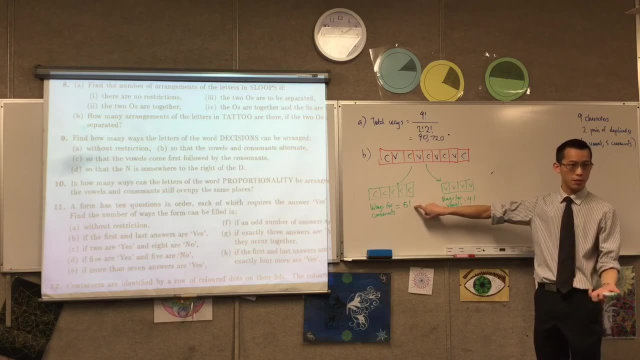 is 4 factorial. OK, OK, now, this doesn't take into account the fact that I've got some repeats. So when you think about the consonants, one of the duplicates is a consonant, but the S's right. 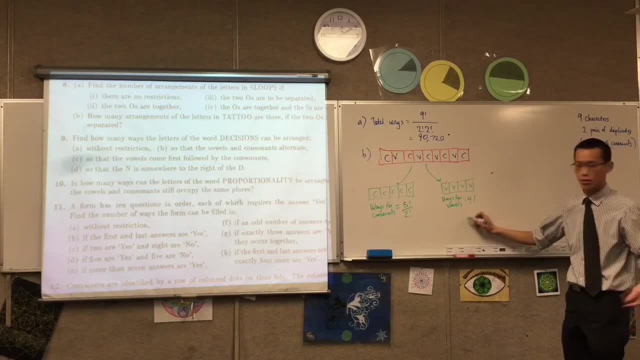 So in fact it should really be that, And then for the vowels, you've got the same deal, right? So there's the I's and that's got a duplicate in it. OK, Now just pause for a moment, because I just 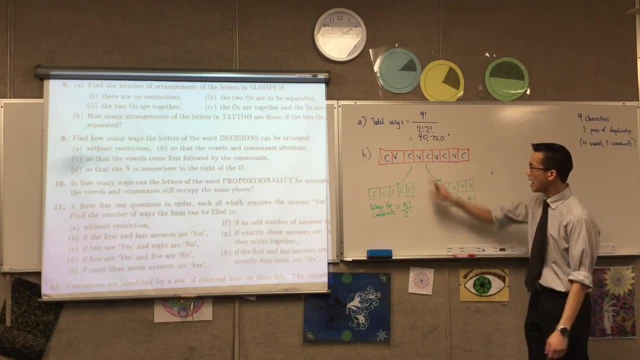 I did something which I don't know. if you noticed like, oh, I can just do that. I pulled out each of these and I said: OK, that's its own sequence and I don't have to worry about where they are. 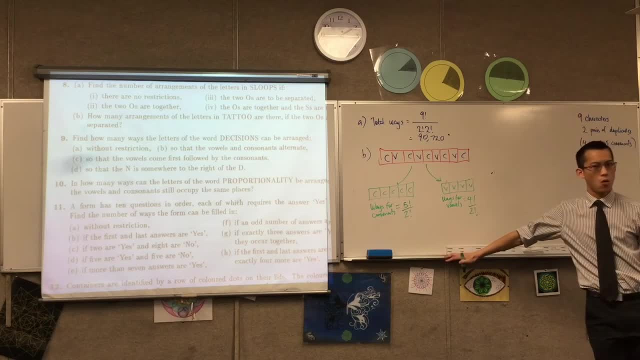 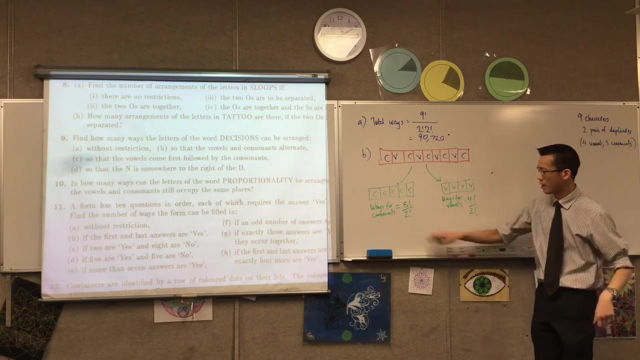 That's its own sequence. I don't have to worry about where they are. Now here's my question: Why can I do that? Why can I just consider this one thing as two separate things? OK, very good. In case you didn't catch that, let me repeat it, and then I'll unpack it a little more. 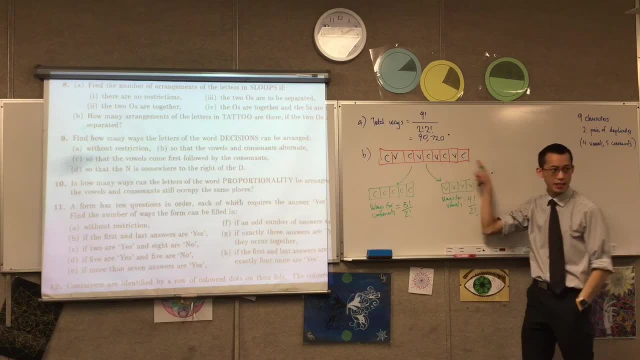 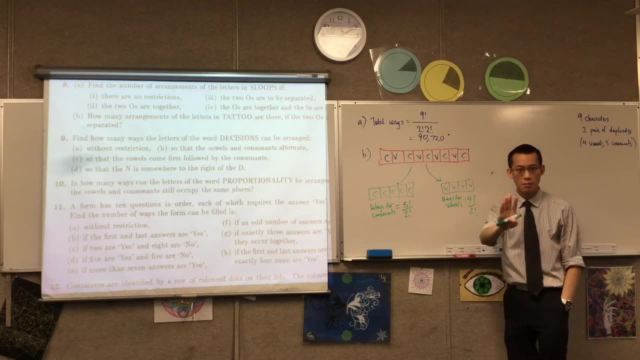 Rash there, which is exactly right. there's only a fixed pattern for how these guys can actually slot into these spots. right, The consonants have to be in exactly those spots. Mark this. there are no choices. I can't choose where the consonants 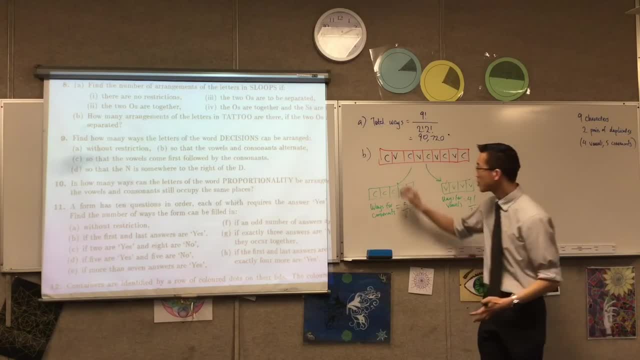 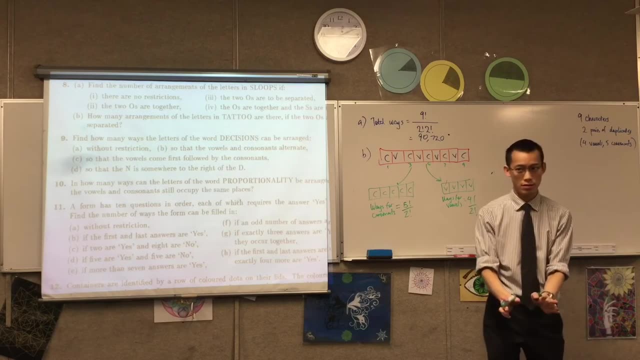 which spots they're going to occupy. Good morning, They have to occupy spots 1, 3,, 5,, 7, and 9, right, There's no other spots they can occupy. There are no more choices And this is why I asked at the beginning, before I drew this box, right. 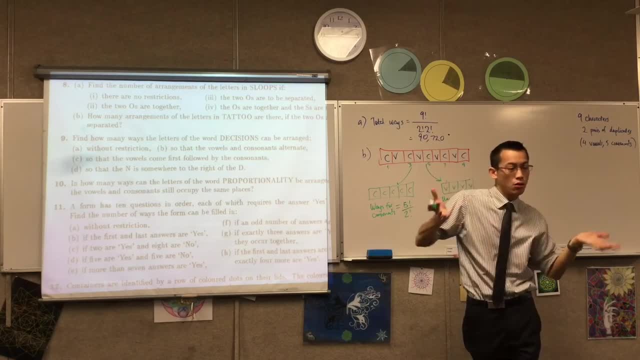 Before I drew this box, I asked: can I start with a vowel Or can I start with a consonant? And you all replied to me: no, you must start with this guy, right? So there are no more choices, right? 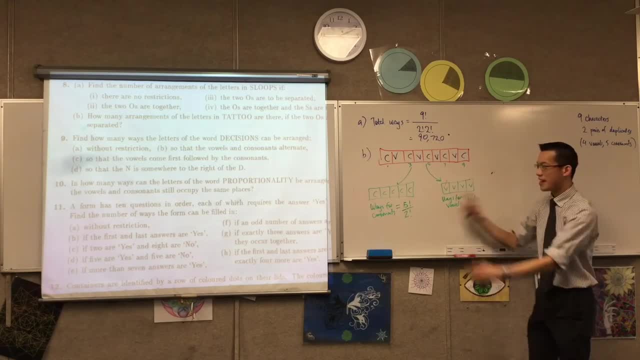 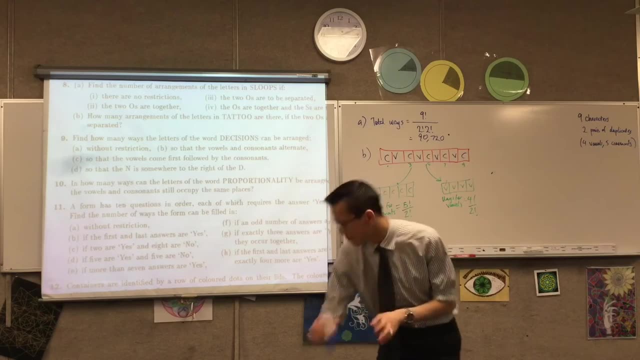 So once I've locked that into place, then I just have to work out the order within the slot. Okay, And that's where this comes up with. And so now I can say the total weight. How am I going to combine this pair of numbers? 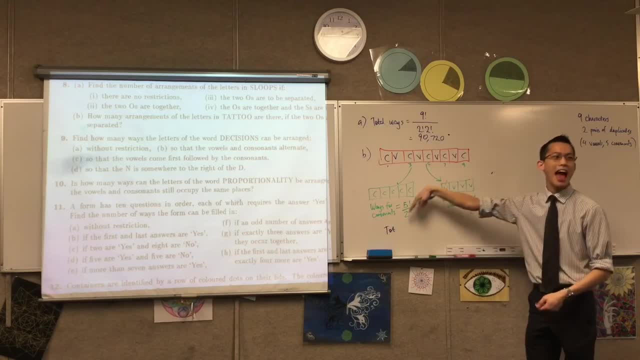 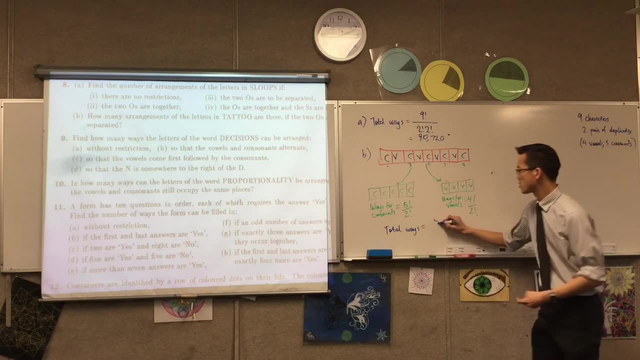 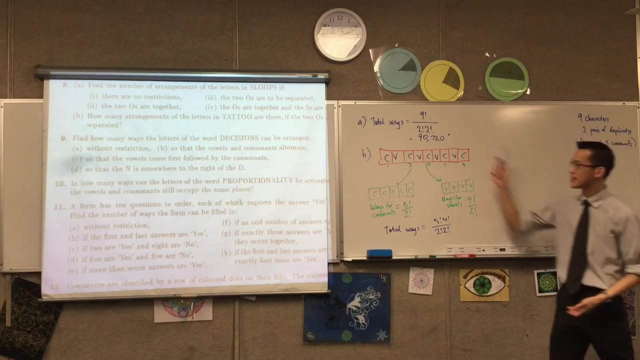 I'm going to multiply right, Because I need the consonants and the vowels together simultaneously. So the total weight is 5 factorial- 4 factorial on 2 factorial, 2 factorial. Okay, Now, what's lovely about having set it up like this is now look at part C. 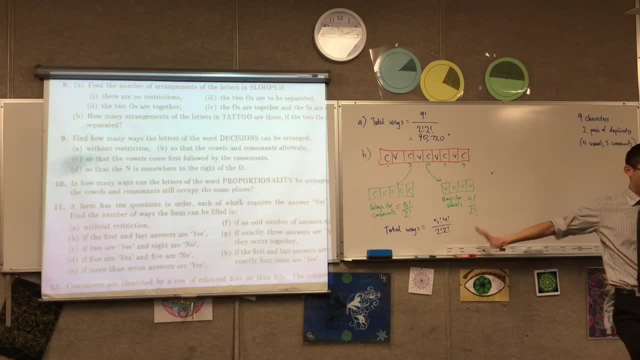 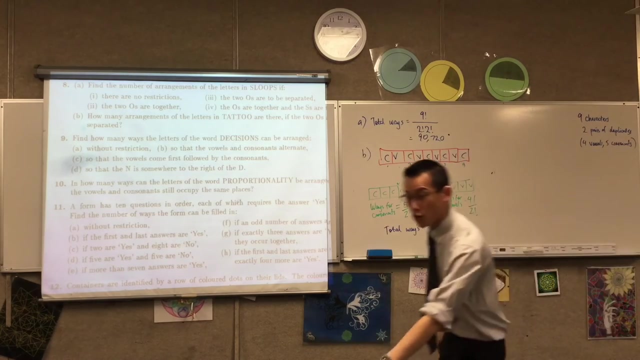 Part C says: arrange the same letters so that the vowels come first, followed by the consonants. Now think about what's similar about this and think about what's different. Okay, Obviously, I can't use this diagram, can I, Right? So I'm going to draw a new one. 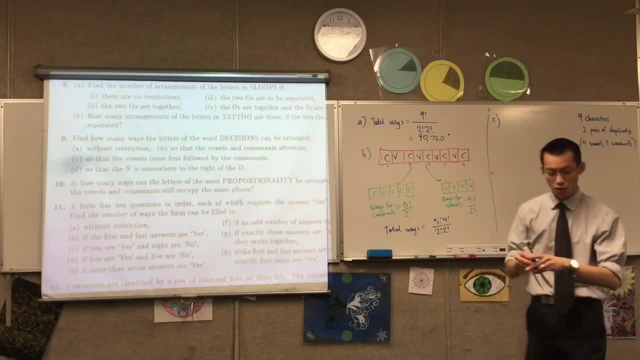 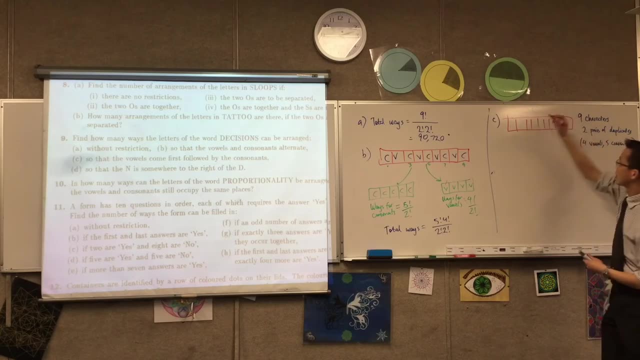 This is part C. I'm going to draw a new one. Still have 9 slots. Okay, There are my 9 slots. I think Did I get 9?? Yeah, I think so. Having a look at this, it's not C, B, C, B, C, B, da, da, da, da da. 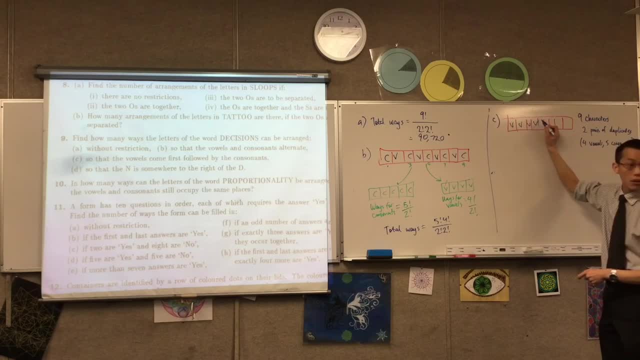 The vowels come first Right. So vowel, vowel, vowel, vowel, All 4 of them, And then the consonants 1,, 2,, 3,, 4, 5.. Okay, Now let me ask this again. 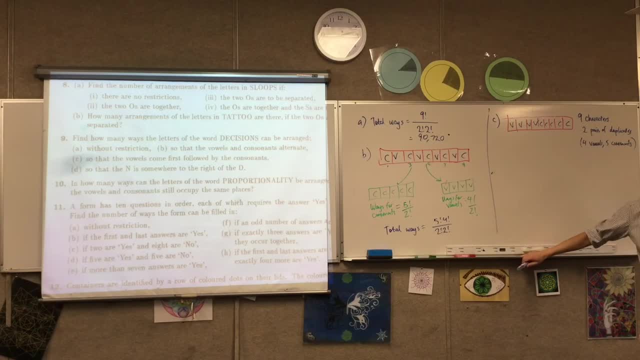 Are there any other arrangements for the vowels and consonants? Answer: no, because that's all they've said, Right? None of these vowels can sneak over here, None of the consonants can sneak over there. So I have no more choice. No more choices. 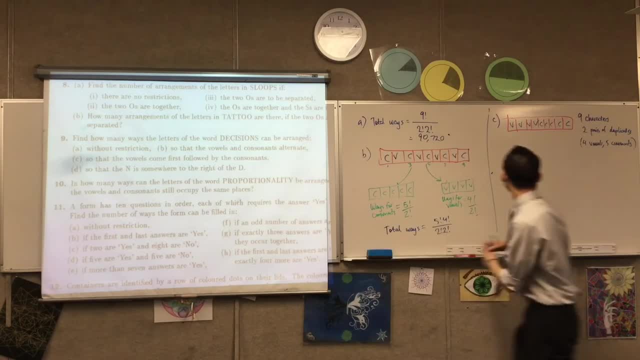 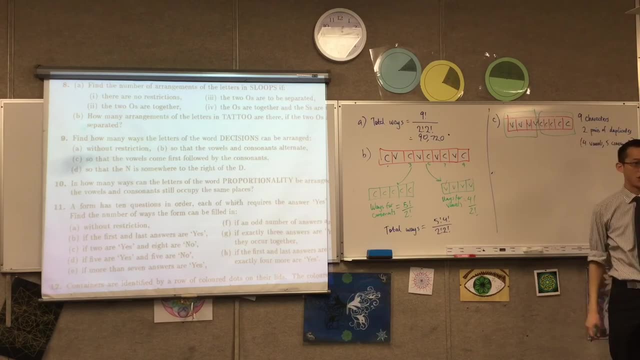 And then I say: well, think about these guys as one, Arrange them. And then think about these guys as one And arrange them, Which we've already done. Do you see that? So, even though this looks different to this, if you can see through, they're the same question. 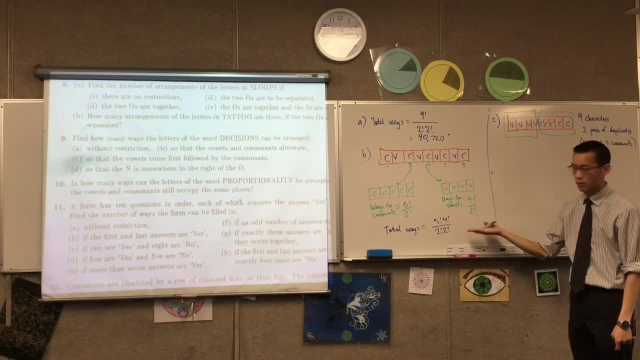 You still have to arrange consonants, You still have to arrange vowels, But you don't have to arrange them with each other. There's only one way you can do them. So there are no more choices. So I don't have to multiply any of these numbers by anything. 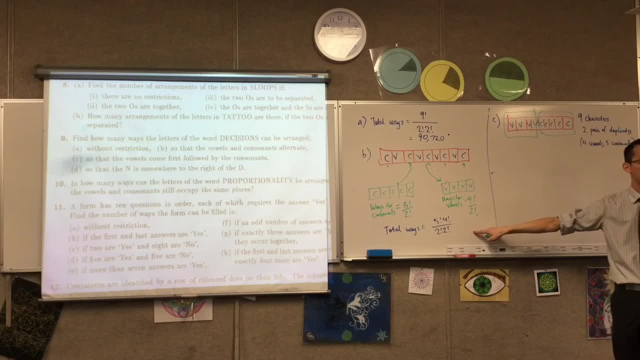 Part C: same answer. Does that make sense? And there's the same number. If I wanted the consonants first and then the vowels, or you get the idea. Okay, All right, So that was A, B and C.